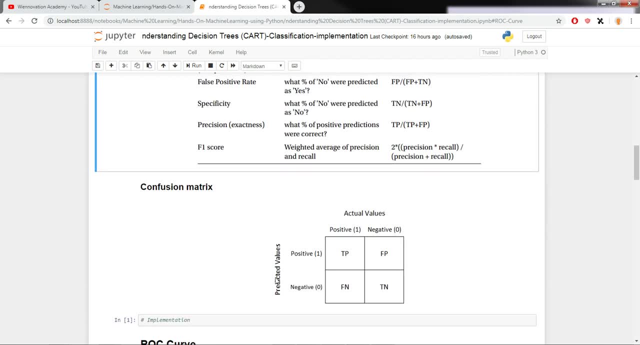 So, first of all, we need to understand what confusion matrix is Before we can actually move on to the much more important and complicated part, which is the ROC curve or AOC. it's important for us to understand what confusion matrix is right Now. what is confusion matrix? Confusion matrix is simply just another matrix, except for the fact that you will be creating an n by n matrix. What is n by n matrix? What do I really mean by the n by n matrix? Well, it means that, so let's say, we had this decision tree. 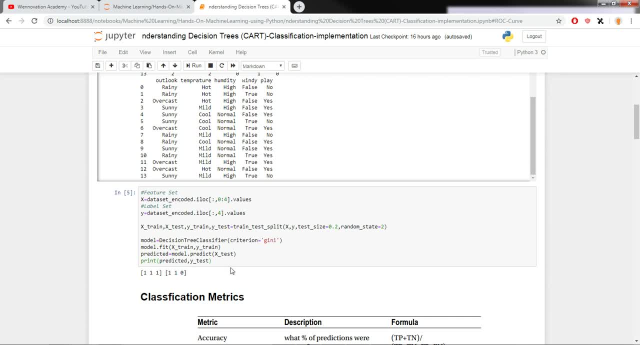 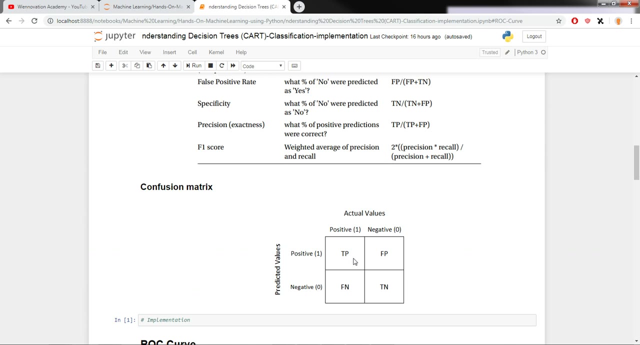 that was predicting ones and zeros, right? so we only have two classes, which means that our confusion matrix will be of two by two, right? so we have two classes. so we need to actually create a two by two matrix. So our matrix will look like this. but let's say our model was predicting, you know, it was giving answers out of three classes. so let's say it was a multi-class classification task. so our confusion matrix will increase by three by three and then it will be a different, right? So right now, let's try to actually understand what this matrix is. 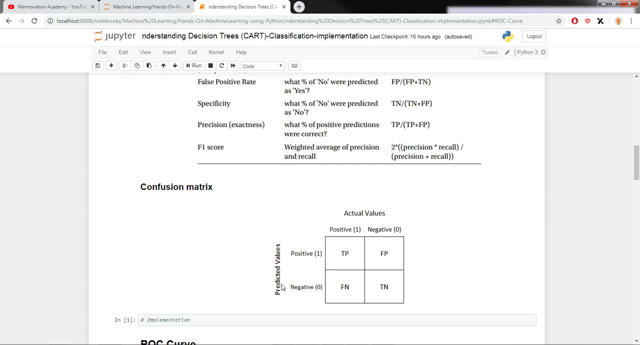 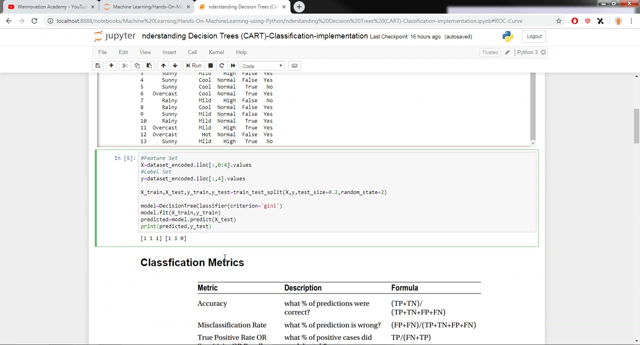 First of all, we're going to go ahead and write positive and negative on the y-axis and it's going to say all the predicted values that our model predicted. right? This is the answer that our model predicted. It can be either positive or negative and, similarly, we have actual values. So actual values are either one or zero, so that is the one that we are using. So this is the y-test right here. These are the actual values of our data set. right? These are the actual values and 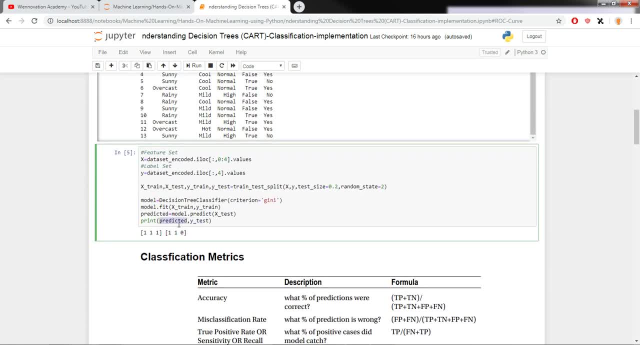 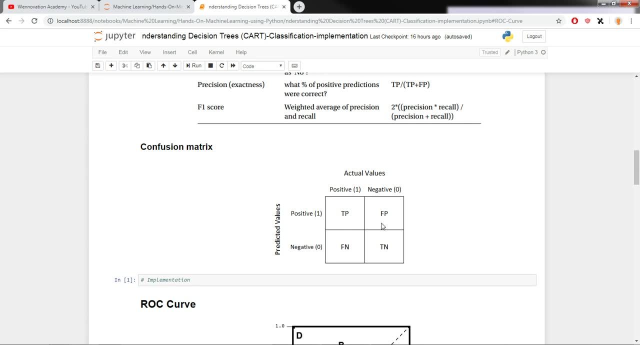 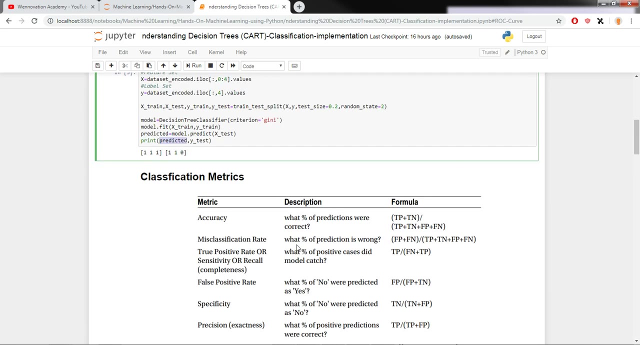 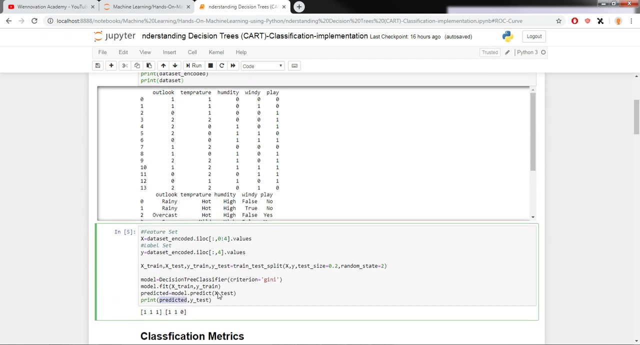 that is, and that is the predicted one. that is our model. that's what exactly our model is going to predict, right? So now we can just go ahead and count those values and we can just go ahead and put them and keep increasing the count until we get a final confusion matrix. This is exactly how we actually go ahead and create a confusion matrix. Now, what would happen if you could create a confusion matrix for the model that we have created right here? right, Let's just do that. So I'm just going to go ahead and see So surprisingly in Python. 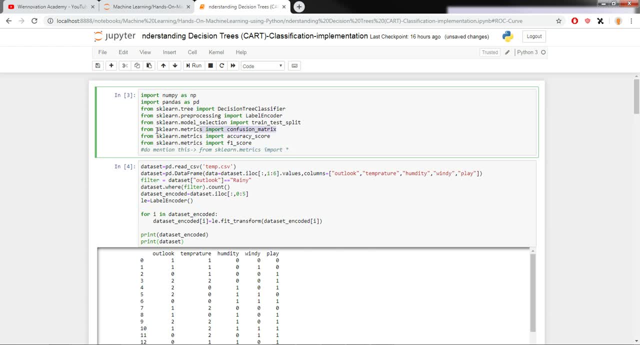 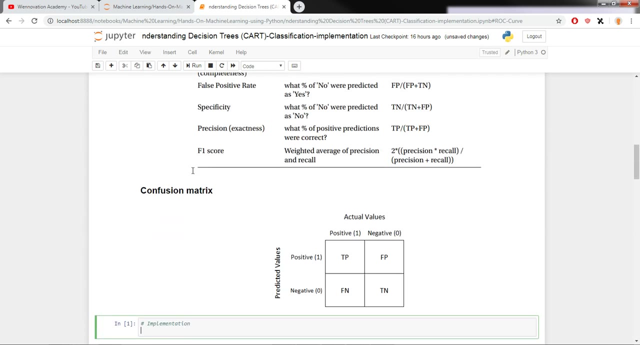 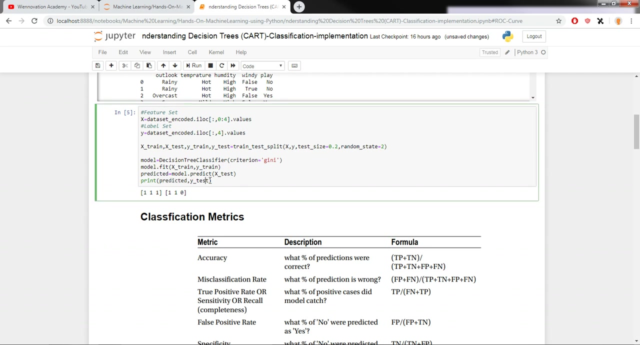 we have confusion matrix built in using the scikit-learn library. so you can use the matrix library, matrix class from scikit-learn and you can directly just go ahead and just go ahead and print the confusion matrix of your model. So I'm just going to go ahead and do that and we need the predicted and actual attribute for that. So we have predicted and actual, So you can just go ahead and put them directly inside our confusion matrix. So I'm just going to go ahead and say 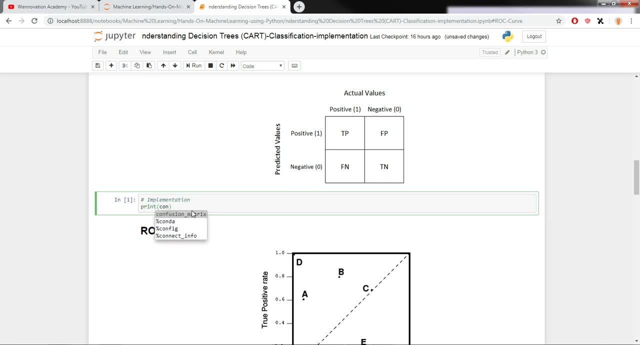 print and confusion matrix and then we needed to write this separately. so because obviously the format of this is, if I press shift and tab, you can see that it says that you need to put a y predict after the actual value. so that's exactly why I need to put a y underscore test before predicted. 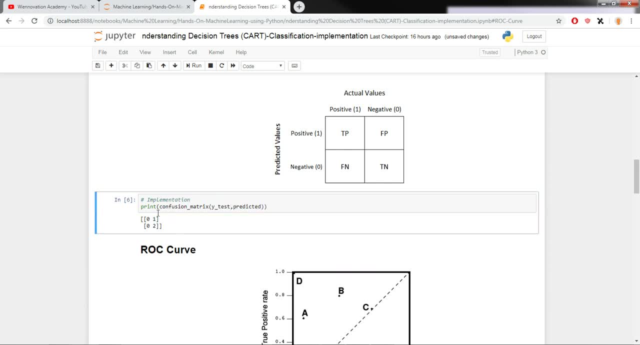 right. so if I just go ahead and predict this now, you can see right now it instantly gives us this answer and from this answer you can kind of get the idea that the true negatives are two and the false part is positive is one. so our true negatives were, let's say, our true negatives were two and it. 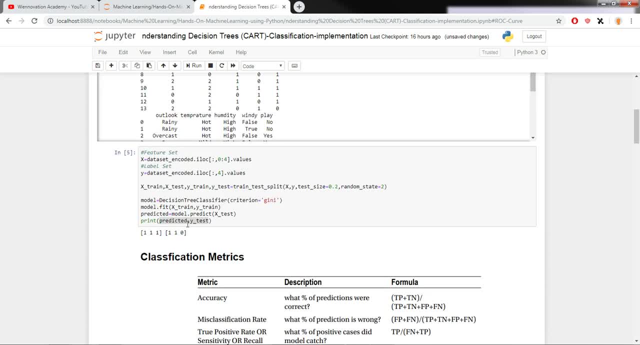 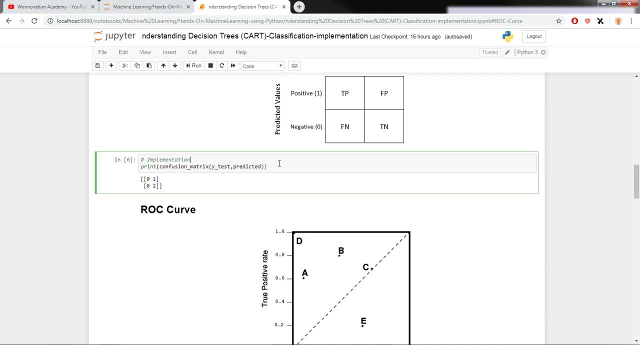 predicted it rightly, and one of them was actually wrong, and this is exactly what you can see here. so you can see, the two of them are right and one of them was wrong. right, so this is exactly what our our model tells us. our model is basically capable of doing it and, secondly, we can actually 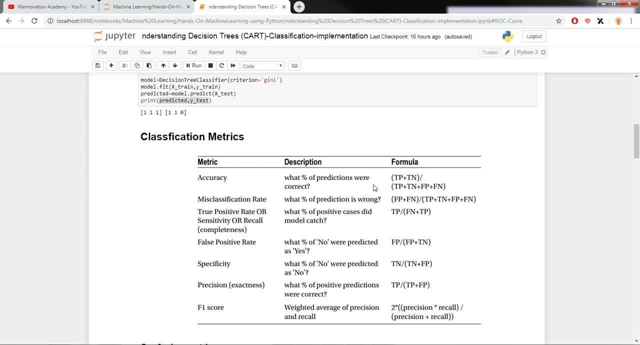 go ahead and calculate the accuracy of a model. so how do we calculate the accuracy? well, we can just calculate that by two positives plus two negatives, divided by two positives plus two negatives, plus false positives plus false negative, and we can just go ahead and put that, put that in a formula and we can directly get this answer. but 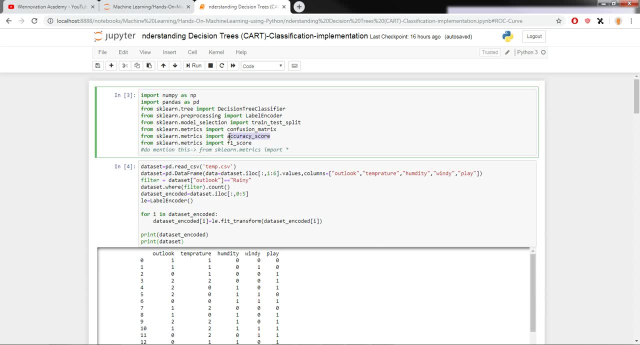 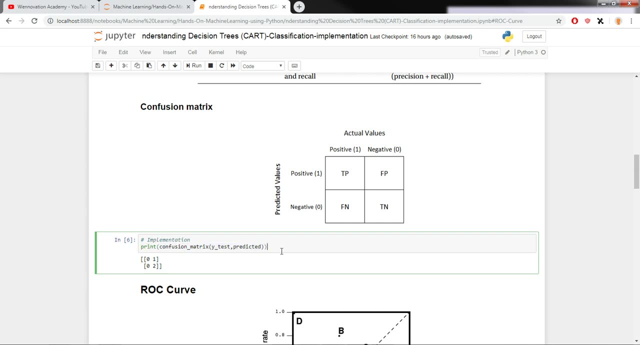 surprisingly, in Python we have that as well, so we can just directly use this accuracy score for finding that out. and how do we do that? well, we can. basically, we can just simply just copy and paste this and instead of confusion metrics, we can just go ahead and write accuracy score. 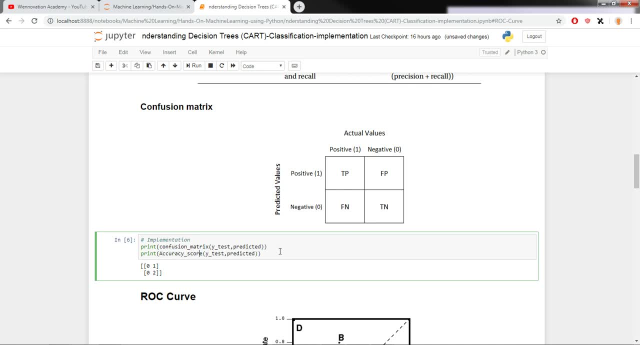 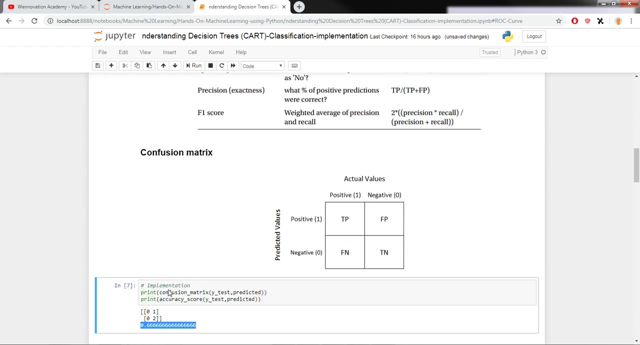 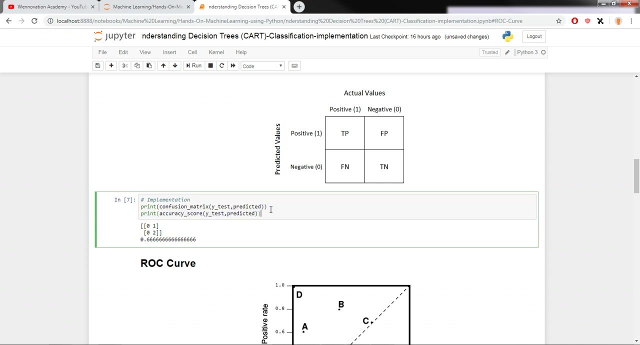 and WALA underscore score and I just put capital here and if I just do this, you can see this is the accuracy score for our model: 60%. this is not that good because obviously our model was not trained that well because we had a very small data set to, you know, for it to train on. so we obviously have to, we obviously need a bigger data and, you know, much more data on which our model can see, and then that's exactly when our model will actually get much more accurate than this right. so now you know. 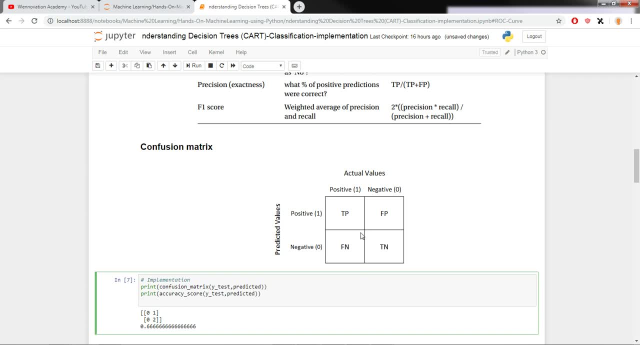 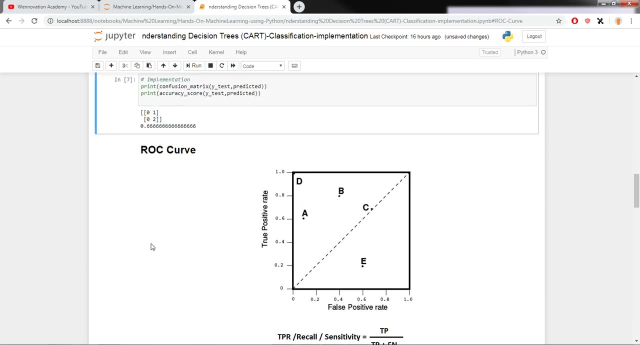 what confusion matrix is and how we can actually go ahead and implement one in Python. we can move on to a much more better- or I can say another- matrix that we can use to actually calculate, or exactly what what basically data scientists use to actually judge a classification model right? so what is an RSC curve? RSC is a probability curve, that that represents the degree or measure of separatability. so what you can say is that you know how do. how can we? 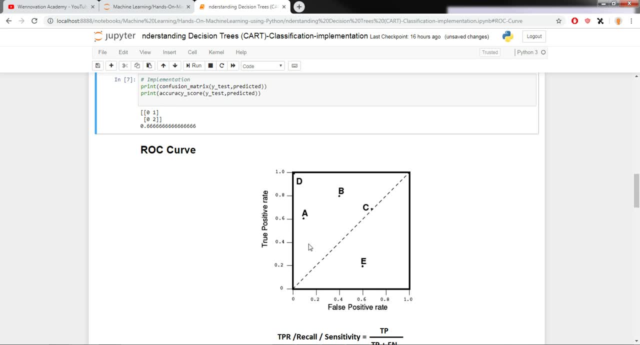 separate our true classes and false classes. so let's say, our model predicted the true and false. so how do we know that our model predicted them rightly? so we can actually visualize that directly using this RSC curve. RSC curve simply just goes ahead and visualizes that for us. so I will actually go ahead and actually tell you what exactly this means. don't worry if you don't understand this right now. right now, if you take a look at this RSC curve, if you take a look at this graph right here, it is simply. we have to simply just go ahead and put a true positive rate on the y-axis and false positive rate on the 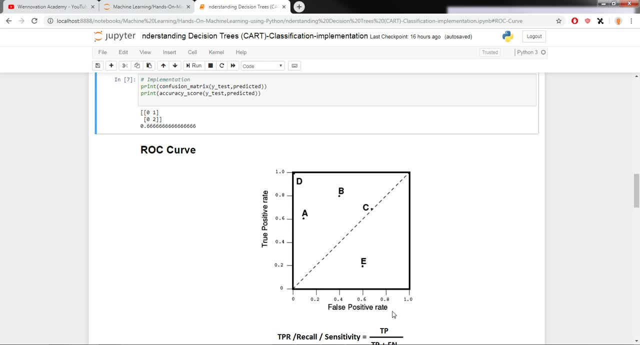 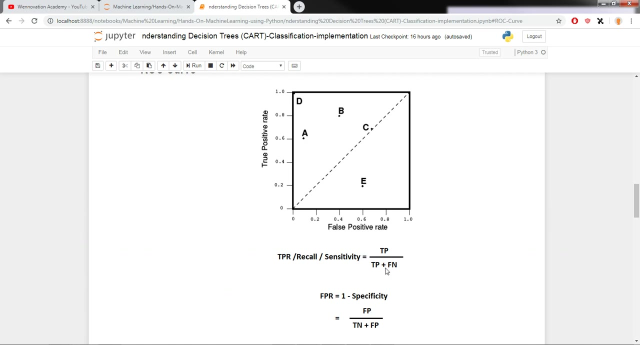 x-axis, and from zeros to one. so that's exactly what the value is from, so that's exactly where the values will vary. so these points are basically the points from true positive rate and false positive rate, and these are the points that we need to plot. and how do we calculate these points? well, simple, we can just go ahead and put the true positive divided by true positive plus false negative, which simply yields true positive rate for us for every instance, and then we need to calculate the same for false positive rate, where we need to put false positive rate divided by the true true negative. 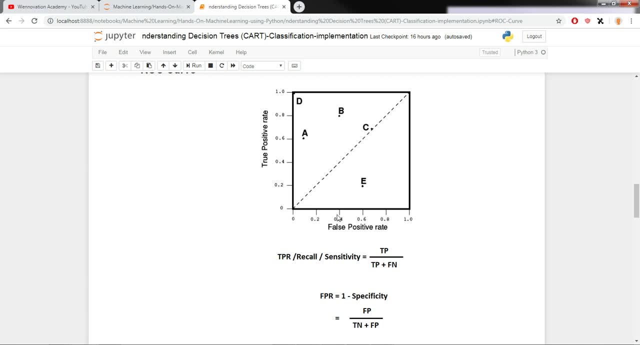 plus false positive, and we get these values for every instance. we get these two values and we simply just keep plotting them until we get all the points of the graph and we simply just go ahead and draw a line over that, and that's exactly how we calculate the RSC curve of our metrics. now, don't worry if you don't understand right now, because I'm actually going to go ahead and show you this in the form of a table and how we can do this. so now, what exactly is RSC? well, the better the model is. so, exactly how do you know that our our so from? how do you? how you can? 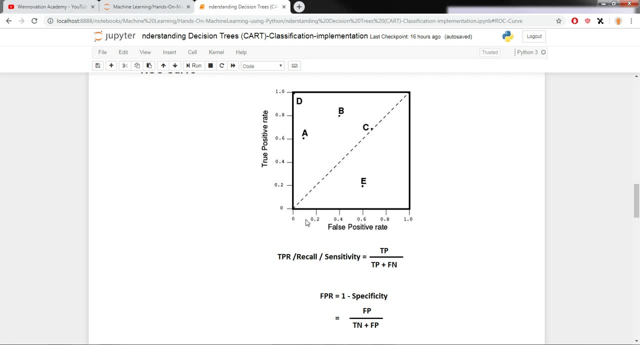 tell, well, whether the RSC was, whether the RSC did the right thing or not. well, our model was accurate or not. how we can tell this by using the RSC. well, it's quite simple. if you, if you, if the curve that we are getting is going to touch one right here, right, this like zero and one, we can say that our model was able to predict the classes, rightly, but what it means is that the model was able to predict the true as true and the false as false. right, let's step. 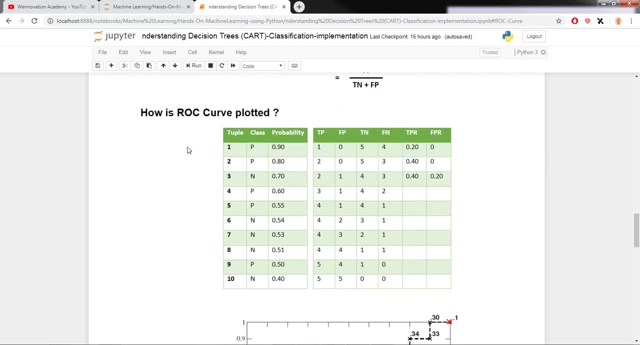 simple, so let's just go ahead and start plotting this, right? so let's say, we had a table like this, so we have a separate sensor. this is like the result that our model has returned, right? so let's say: this is the result that our model predicted and let's see if. whether this model, whether 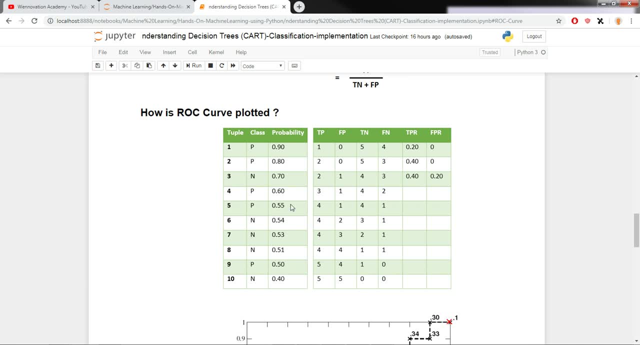 whether this is right or not right. so to do this we can just go ahead and count the number of positives or negative. so the two positives are. so let's just say we can mark a line right about here and then we can just go ahead and draw a table like this are three positives, four positives, two negatives, false, negative, negative and negative and negative all together, using RSC to check that all of those results. 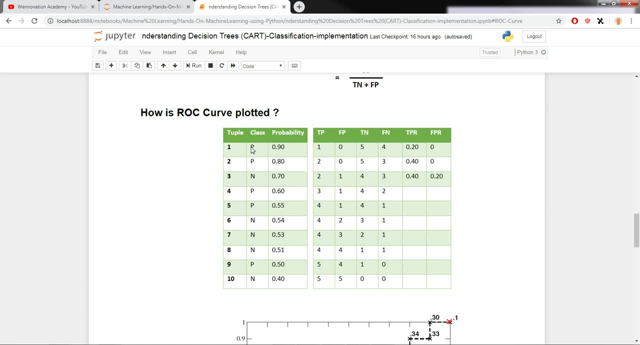 and then we can just go ahead and count it. so. so how many true positives are there? so what our model predicted and what is actually is true positive, that is one. and what about the false positives? well, there is none, because we are marking the right, we are marking the line right. 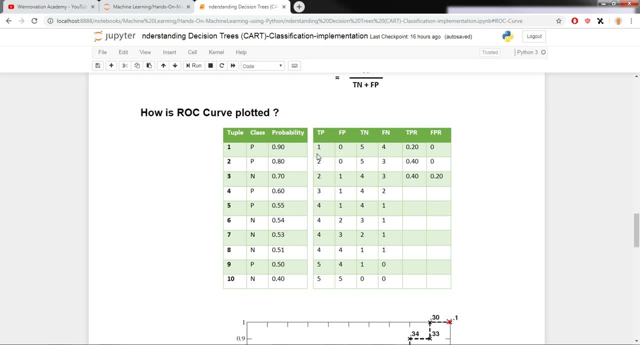 about here. so there is none. so we can just go ahead and put zero right and then we can just go ahead and check the all of the answers beneath the line, beneath this, this marker right here, this is an imaginary marker that we have. we are assuming, like that's right here so we can just 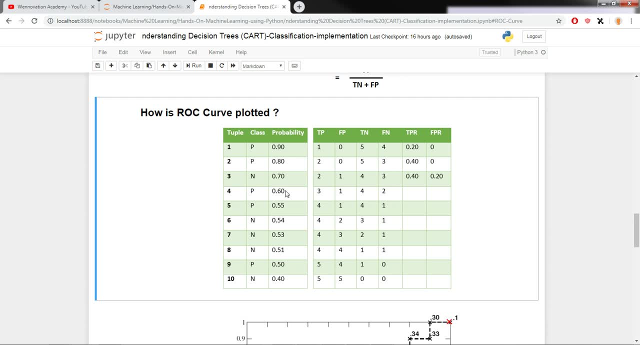 go ahead and count the number of true negative. so how many of them are negatives and they're actually negative? so we can say one, two, three, four and five. so you would put five here. what about the false positive? what about the false negatives? well, the false negatives are three. 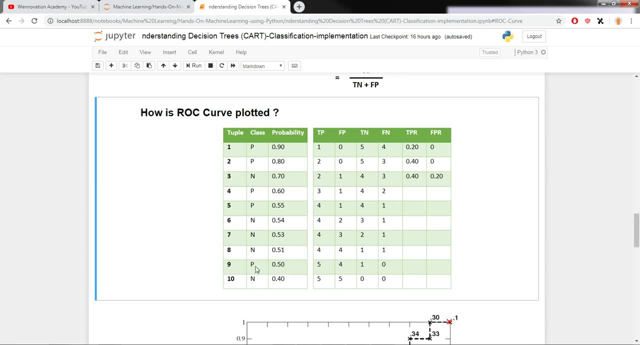 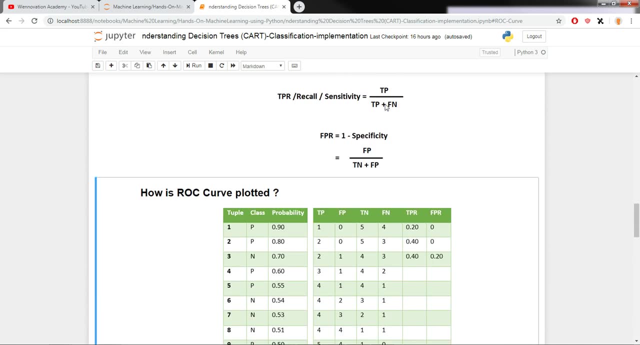 because we can count them. we can see one, two, three and four, so you can just see that that that is exactly what we have, four right. and then we can just go ahead and use these formulas that i've showed you above and we can put these uh values in these formulas and 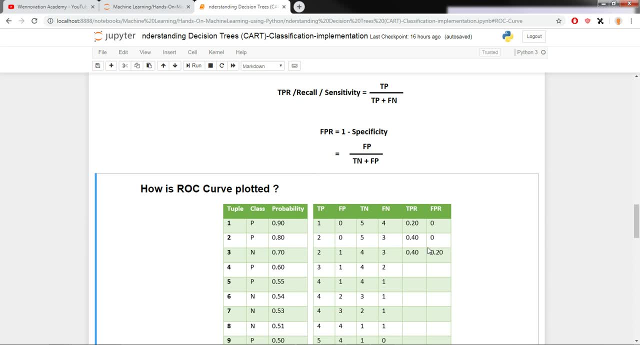 you can just go ahead and use these formulas that i've showed you above and we can put these. you're going to get these values 0.200, 0.40,. you can calculate this Now. I'll leave this as an exercise for you guys, so you can just go ahead and calculate these values. 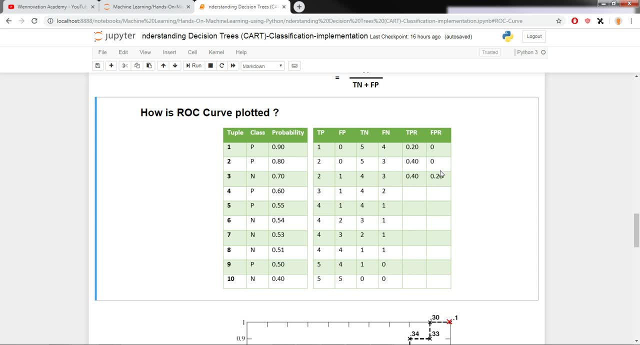 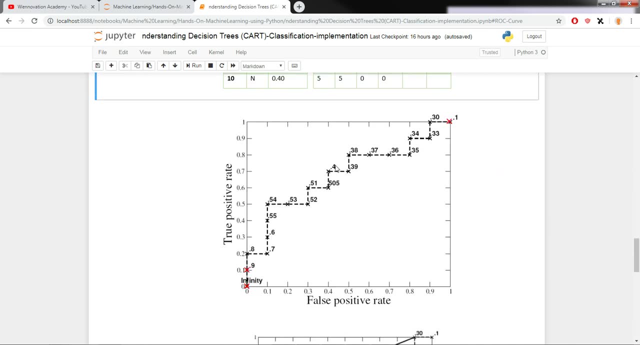 further, and once you get all these values, you can just go ahead and directly plot them similarly to how these values are plotted right here, and you're going to get a graph kind of like this right So now, how do we know whether our model? 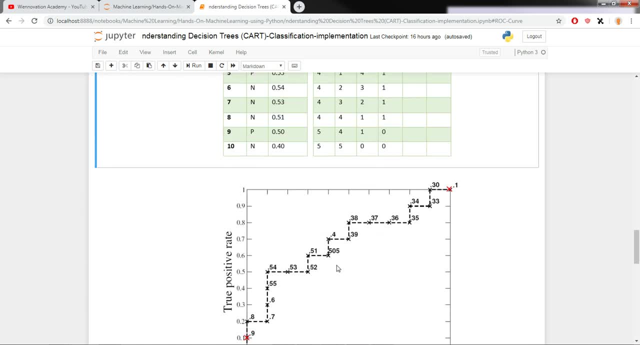 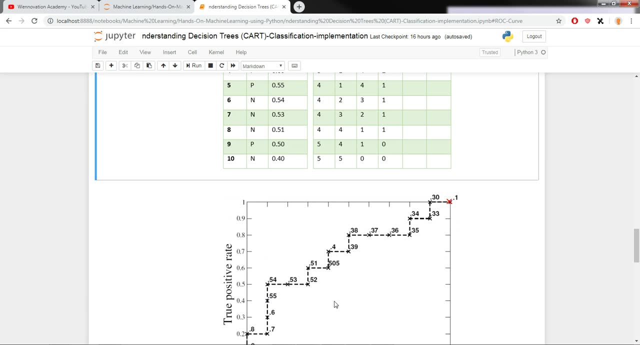 was good by seeing this graph. As I mentioned earlier, the more the graph reaches this point, it means your model was good, right. And the more your graph reaches the diagonal point, which is this line right here, this is the diagonal, so it means that your model 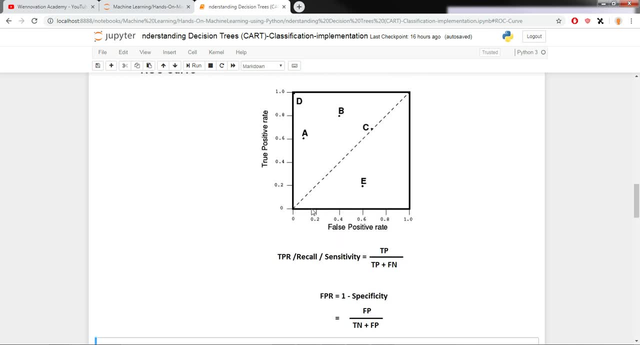 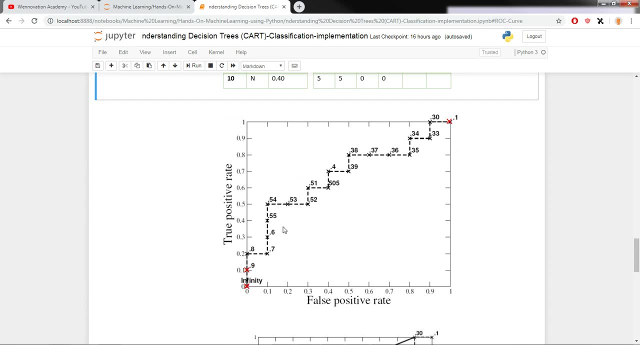 is not good and it's very incapable of distinguishing between the yes and no's right. So from this you can go ahead and see this point right here and you can instantly tell that this is the best our model can get. that's 0.54.. 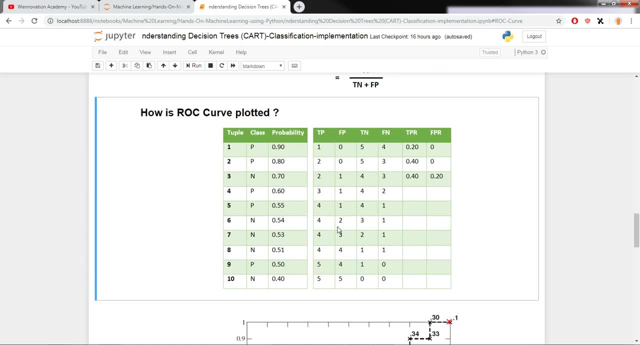 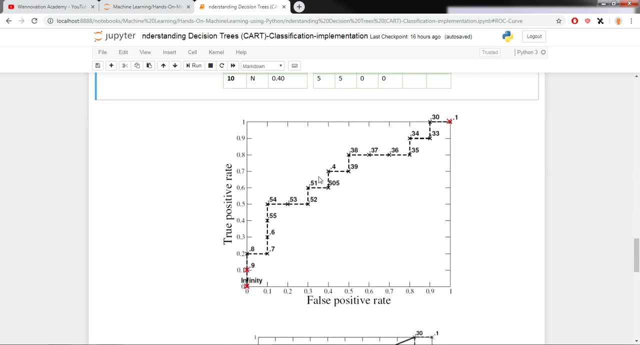 Obviously, this is not the graph from this table and this is exactly why I'm leaving this as an exercise, so you can just go ahead and make a graph or draw a graph for this table right here and check what you get and what is the accuracy that you get from this graph. 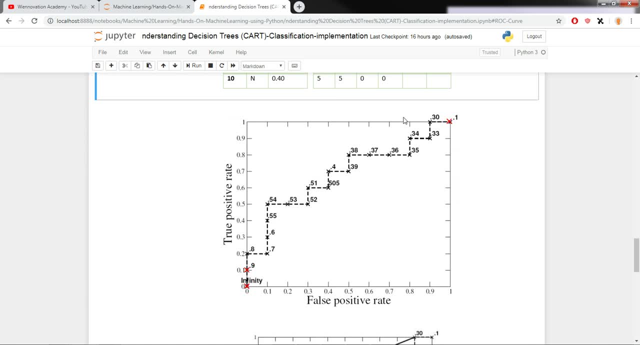 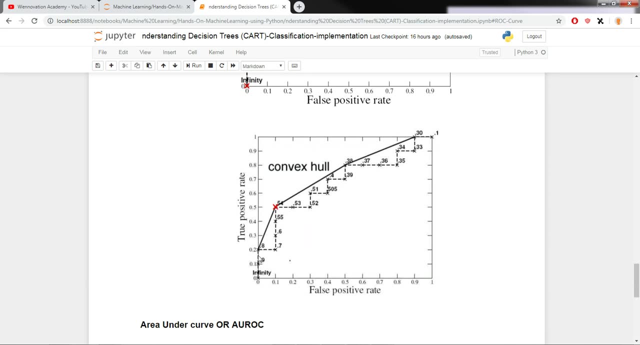 right. And then how do we draw the ROC curve? Right now, these are all the points, and then you just plot these points. How do we draw a curve from this? Well, you can just go ahead and use the concept of point XO, which simply just goes ahead and 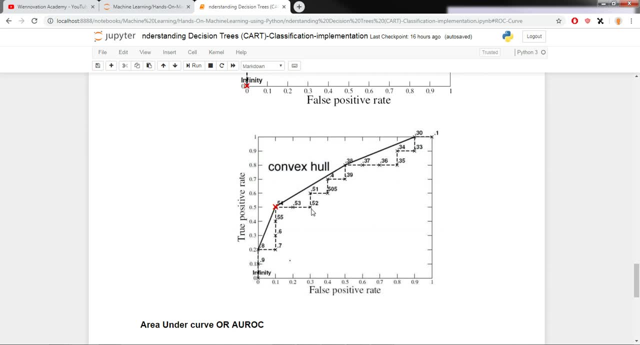 you can just go ahead and pick all the corners of this, or simply the edges of these of these points, and draw a curve like this, and this is exactly what an ROC curve looks like, and you can see that this is the curve that you get right. And now? 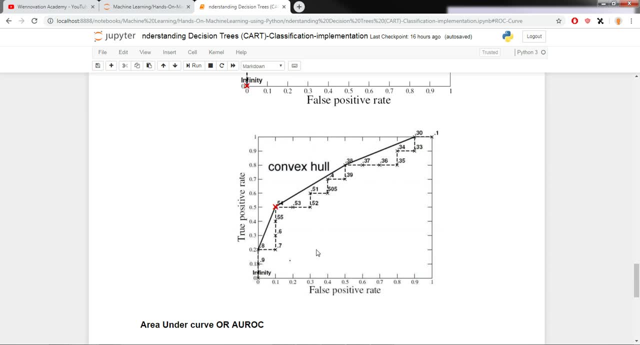 so this is exactly where we come to the point. what is the area under the curve? So the area under the curve is all the area that is inside this curve. So what I mean by this is that the more your point touches this point right here- 0 and 1,, the more better. 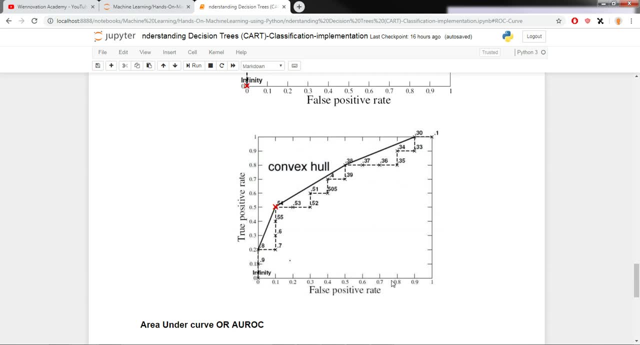 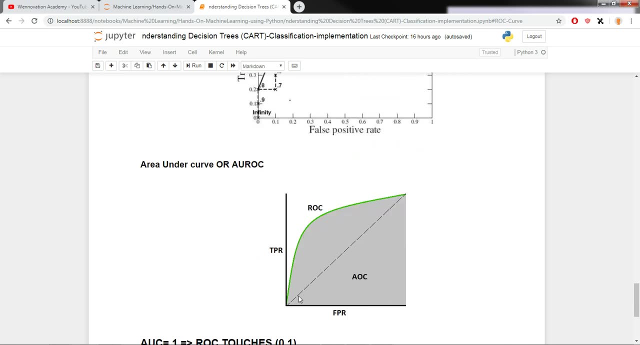 your model is and, similarly, the more area you have under this graph, the better your model is. so this is exactly what area under curve means and you can see uh. so area and the curve is simply the curve beneath your uh, beneath your, beneath your uh. 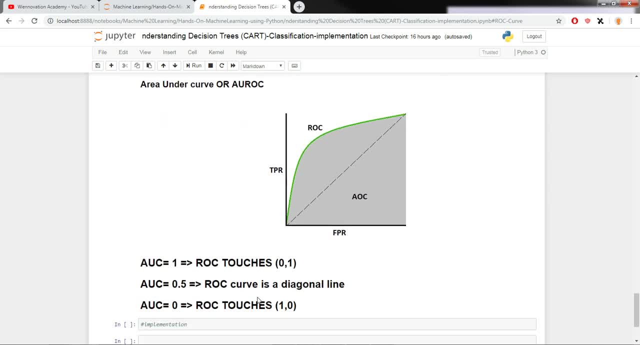 convex hull. uh, curve right here, see, so what do you mean by the aoc? one aoc so what? so what i mean by this is that if your area under curve is one is equal to one, which means that your your roc curve touches this point right here. and similarly, if your aoc is equal to 0.5, then 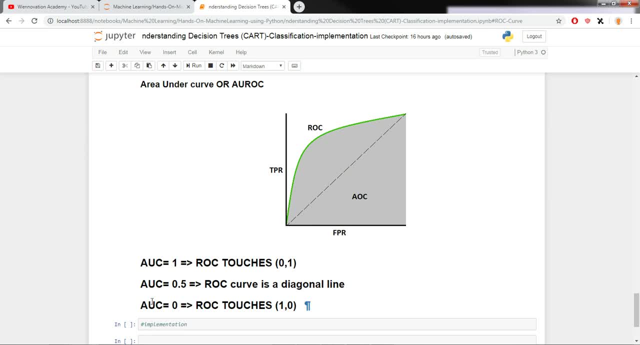 your roc will simply be a diagonal line and if your aoc or area, the curve, is equal to zero, the roc will simply just go ahead and touch this point right here, which means your model was. your model was basically reciprocating the values, so if it was zero, it was predicting it as one. 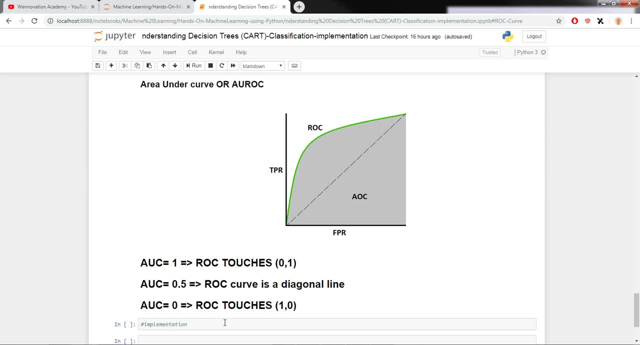 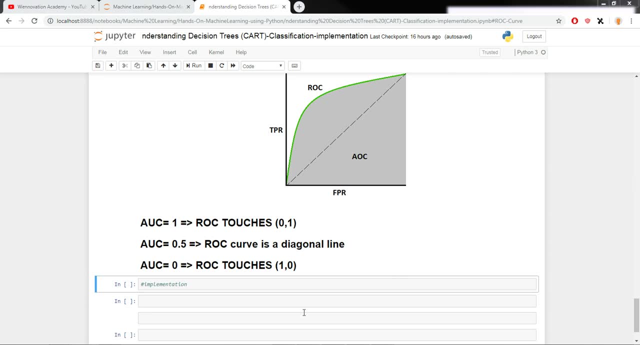 and if it was one, it was predicting it at zero. so this is exactly why ac was zero. so now in python, we're just going to go ahead and implement this right. so, uh, how do you implement this in python, right? first of all, i'm just going to go ahead and, uh, import few libraries. 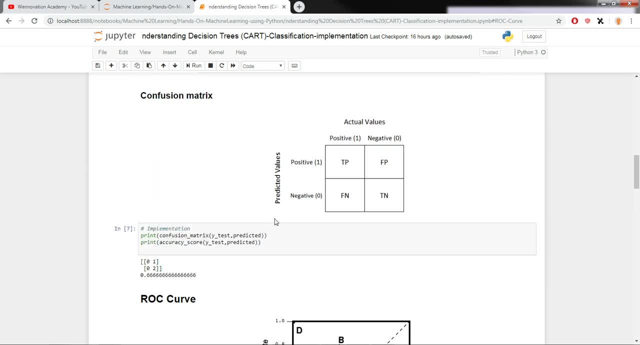 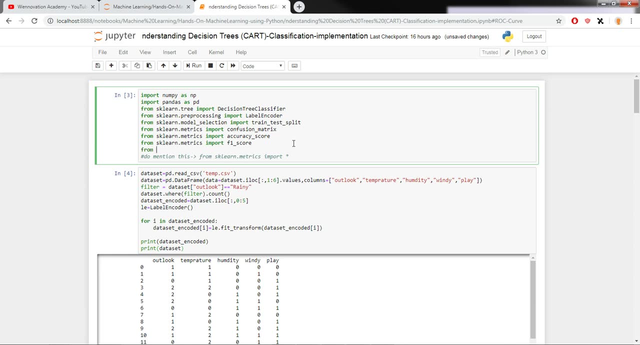 and then i'm just going to go ahead and import a few libraries and then i'm just going to go ahead. i need, i need. so first of all, i'm just gonna go ahead and import an roc curve library from cycle learn, which is a part of how to learn right. so i'm just gonna go ahead and say from um sk learn. 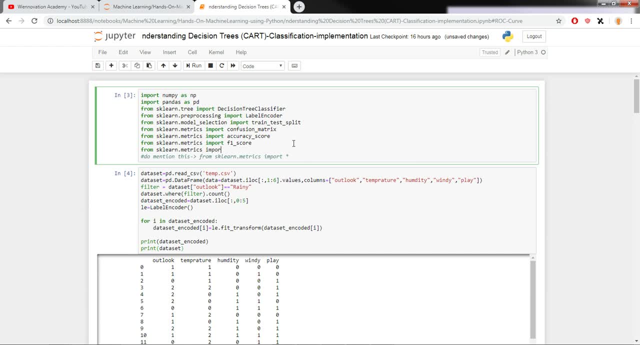 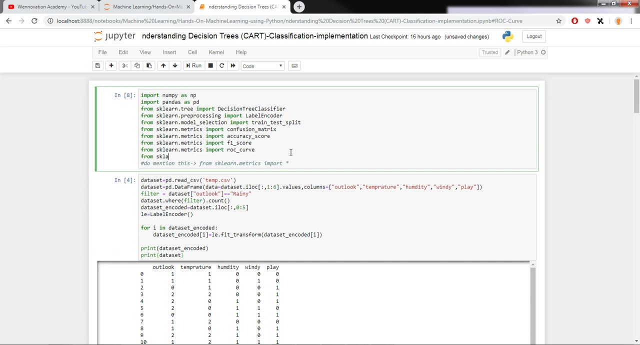 dot matrix: uh, import. you can see roc underscore curve, right? so this is exactly how you import roc curve. and the second thing that we need to import is the roc curve score, because we also need to calculate the score as well. so sk Taylor dot metrics: import ROC underscore accuracy score right. 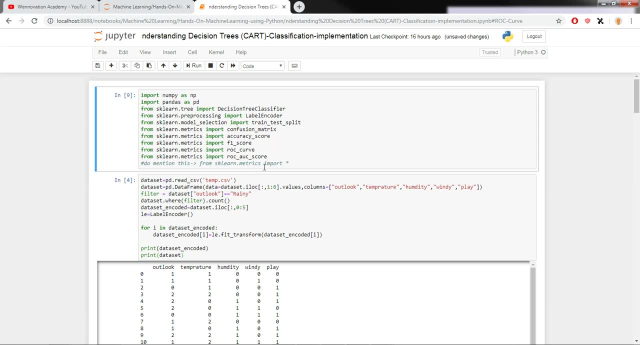 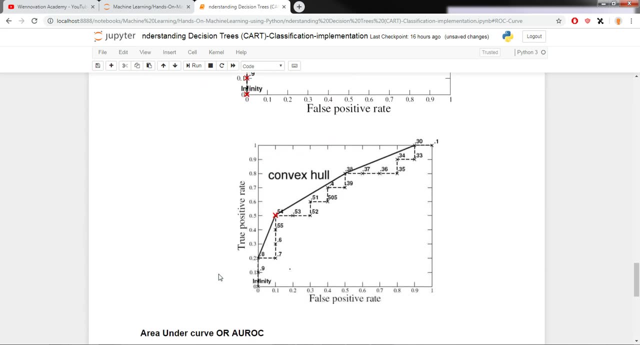 So this is exactly what AOC score means, And this is just going to return an answer in a form of points, And we will simply see how we can use these libraries to calculate our ROC curve or even plot our ROC curve, And this is exactly what we're going to do, okay. 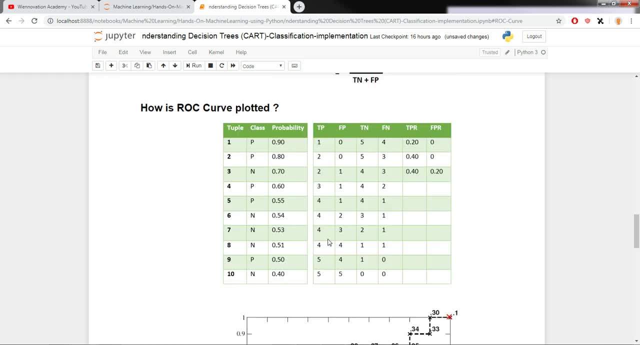 So now we're going to be using the same model that we have right here. So this is the model we have, This is the model I have, So I'm going to be using the same model, right? So how do we do this? 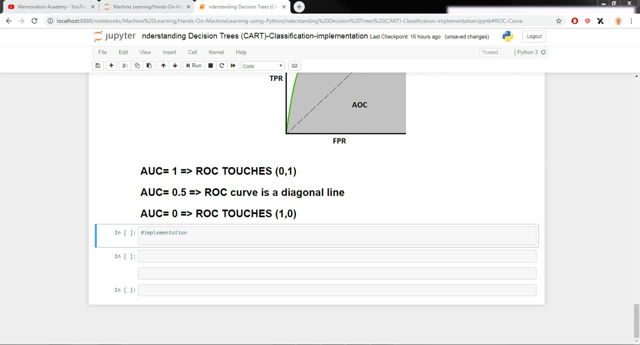 Now the first thing we need to do is going to be pretty simple: We just need to go ahead and simply calculate the probabilities, right? So probabilities equals model dot. So now, model is our model that we created above. So this is the decision tree model. 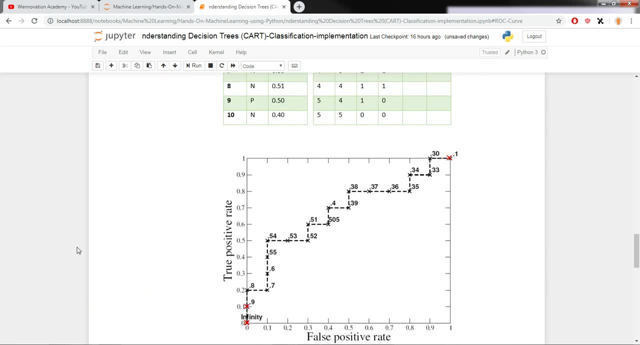 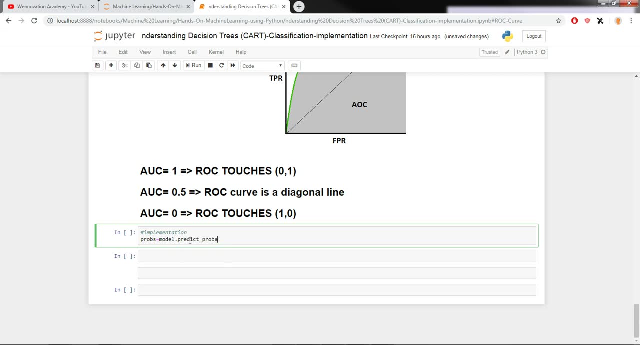 And if we create a C, this is the model right. So I'm just going to say: and then we have a function called predict underscore. so model dot predict underscore probability. So this is simply the function. We just simply I don't know. this function is not the name of the function, is not that good, obviously, but you got to remember that. 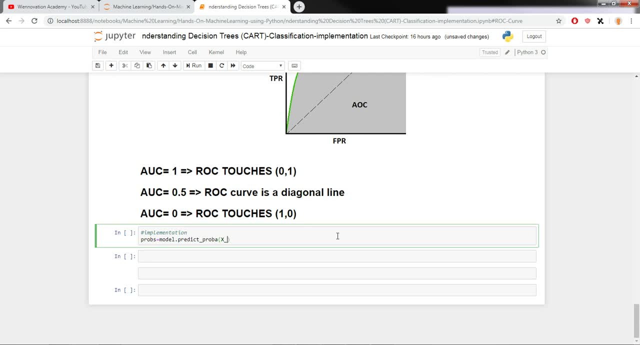 And then we can just go ahead and pass in the X underscore test values. Now, that is the test input, right? So I'm just going to pass this And then I'm just going to go ahead and print this probability. 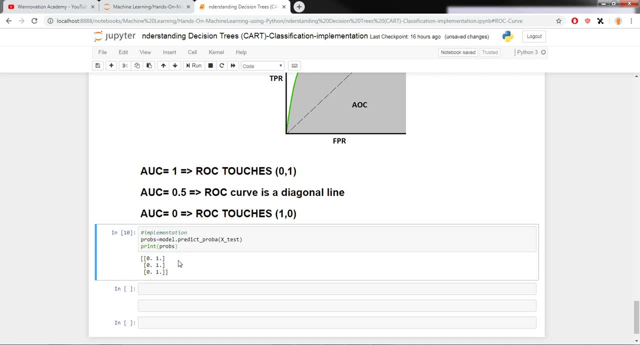 So the probabilities are going to be. So you can see the probabilities for every single, for every single input set that we have is kind of like this: So the probability is 0% and 100%, 0% and 100%. 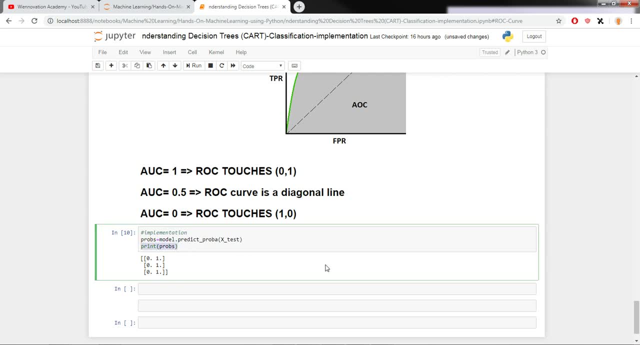 That's how you predict the probabilities, right. And now we can just go ahead and just take, let's say, the first probability of our graph, So we can just say prob equals probs, and we can just say all rows, and I want the 0th probability. 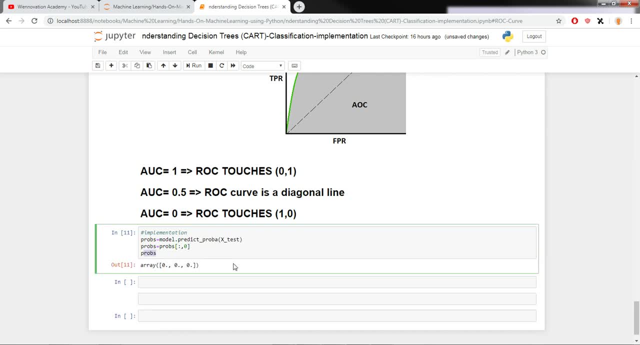 So if I just go ahead and print probability now, you only have the first one. So that's the first one, So that's the first one, right here. And then we can just go ahead. and let's say, I wanted to calculate the AUC score, right? 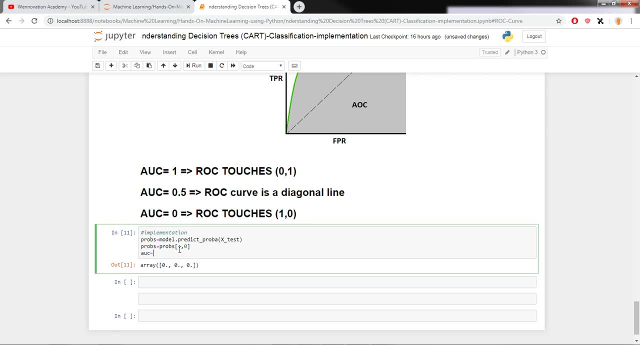 So what we can do for that is, we can just say AUC equals, which is just a variable name, And I can say ROC underscore, AUC score, And then the AUC score receives two things. So it receives the true outputs, which are the actual outputs, and the scores. 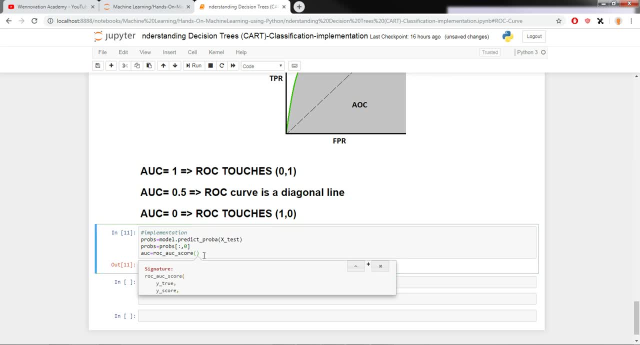 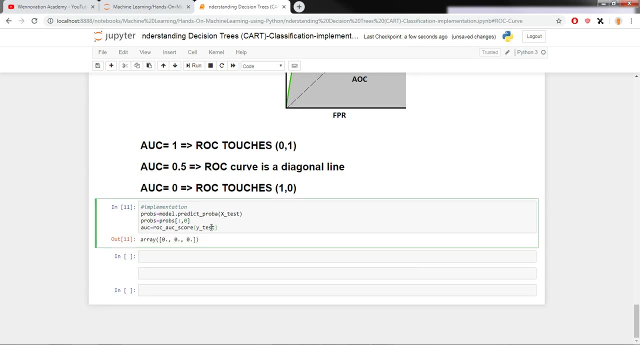 So the probability score that we calculated right here, right, So I can just go ahead and say Y underscore, So I can say Y underscore test, and then I can put the probs that I calculated and this is going to return the AUC score. 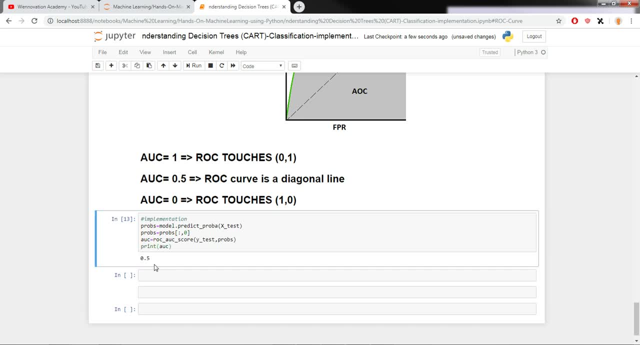 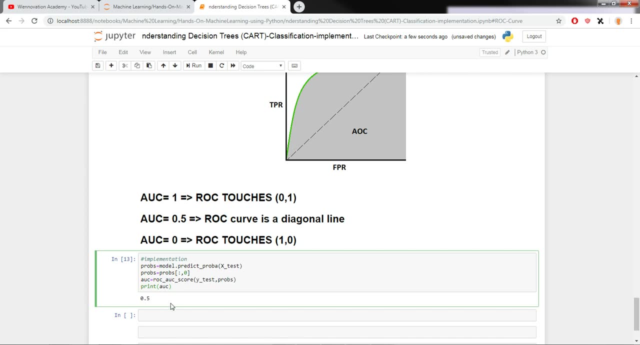 I forgot to print this out, So if I just put AUC right here, you see that the answer is 0.5.. So this means that our model was basically incapable of predicting between 0s and 1s, and it's fairly fair, because we did not give it enough data set to train on. 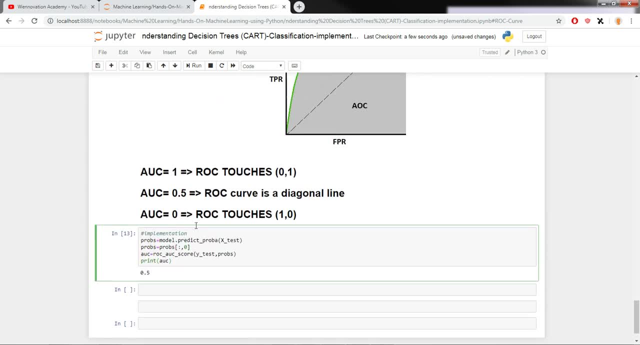 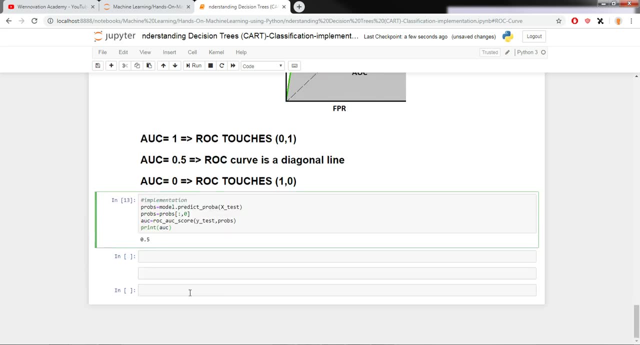 This is exactly why we are getting such a low AUC score, And from AUC score 0.5, you can kind of tell that our model was basically a diagonal line on our ROC curve, And you will see this when we will actually plot this right. 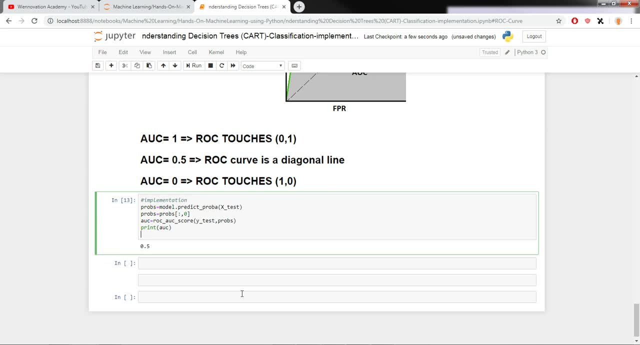 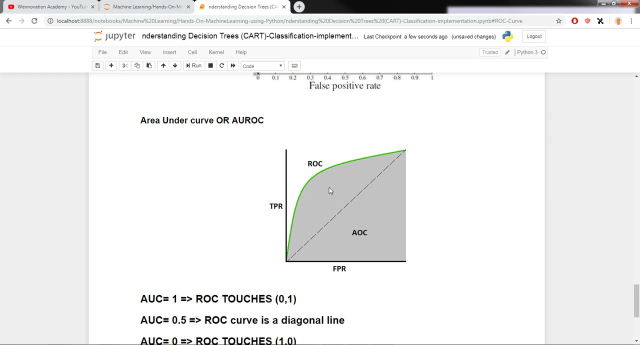 So I'm just going to go ahead and plot this now. So how do we plot this? So, for plotting, you definitely know that we need TPR, we need FPR and we also need the ROC curve, right? 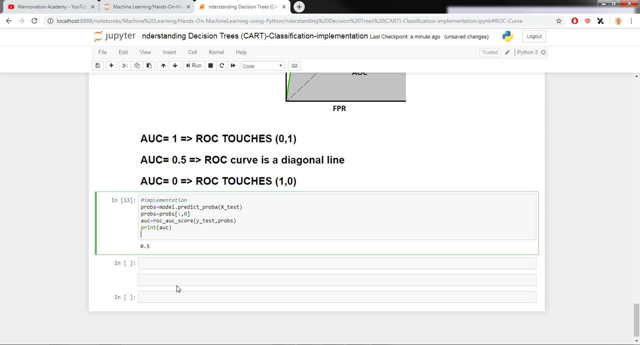 So we need the threshold, we need the TPR and the FPR, right. So I'm just going to go ahead and do that. So for that we can just go ahead and say FPR equals TPR, comma TPR and simply the TPR. 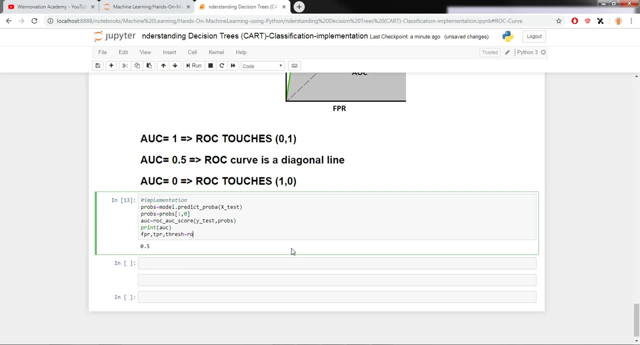 So I'm going to call that as threshold. so I'm going to call that as threshold and equals ROC curve, which is a scikit-learn function, that's a predefined function, and this receives two things: First of all, it receives Y underscore test and it also receives the probabilities right. 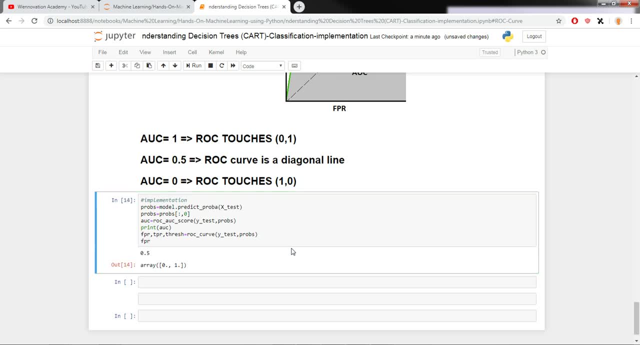 So we just go ahead and put the probabilities right here And now. if you just go ahead and print it, just print out the false part as a positive rate, you can see that it just completely goes ahead and calculates exactly the table we needed. 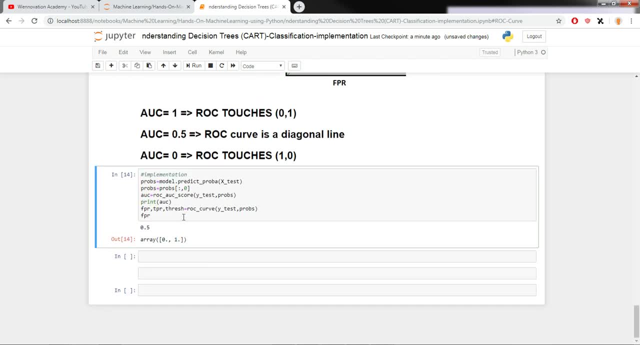 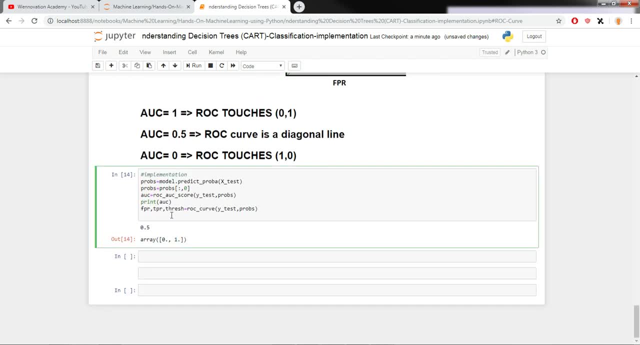 So this is the table that we wanted, right? So now from this you can kind of tell that we can just directly put them in a graph and it's going to just go ahead and print the probabilities for us or simply print the ROC curve for us, right? 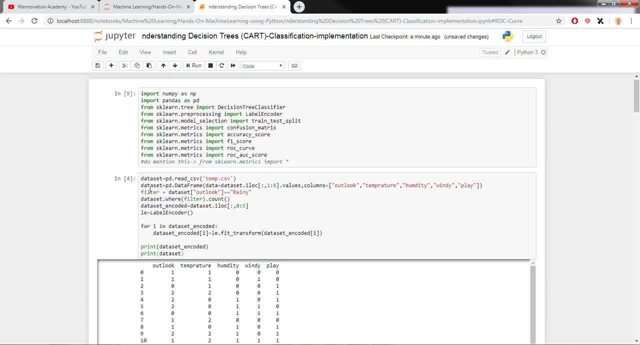 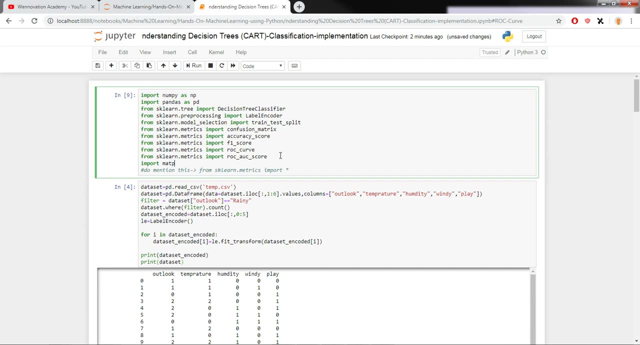 So I'm going to use the matplotlib library. I hope that I have imported that. No, I haven't imported matplotlib, so I need to first import matplotlib. Import matplotlib, dot, pyplot as plt right? So if I just import map for lib, it's going to take a little bit of time. so we have now. we have imported this. 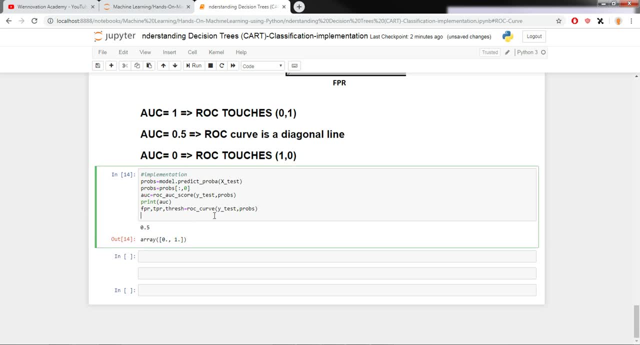 we can go down, and now i'm just going to go ahead and say: well, simple, plt, dot plot, and first of all we need to draw a diagonal line. so we're going to draw a diagonal line from zero to one and we're going to also draw a line from zero to one which approaches one and zero. right? so this is exactly. 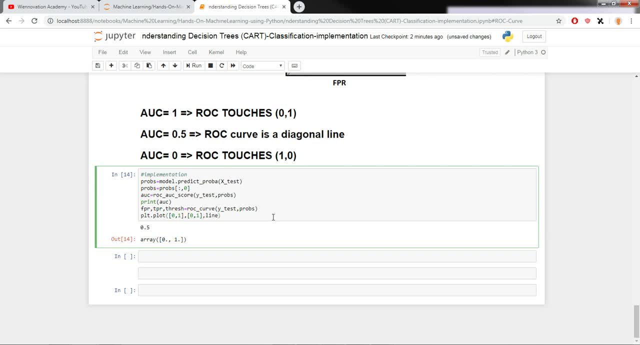 what i'm going to do, and then i can say: well, since i want to draw this, so i want to draw this in a form of dotted lines, right, so i'm just going to go ahead and draw the dotted line, so for that i can just go ahead and put a style as dotted right? this is exactly how you draw the line, right. so if you 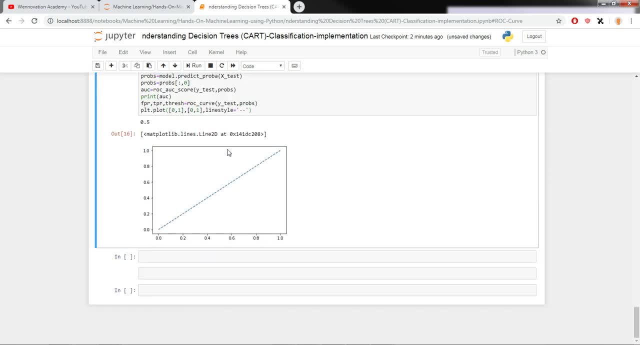 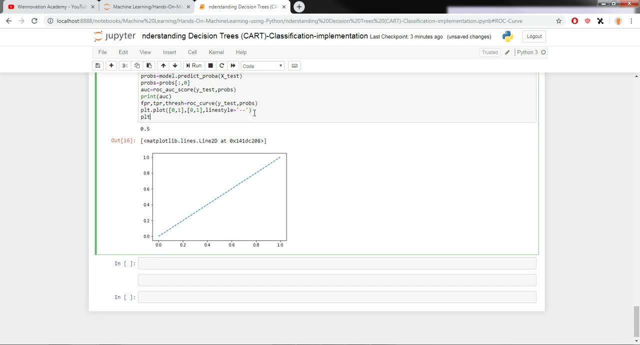 do this. you can see that i have a perfect line right here and now. we can just go ahead and plug our f- the false positive rates and true positive rates- on this graph right. so for that i what i need to do is i need to say plt, dot, plot, and well, what we need to do? we can just go ahead and say: 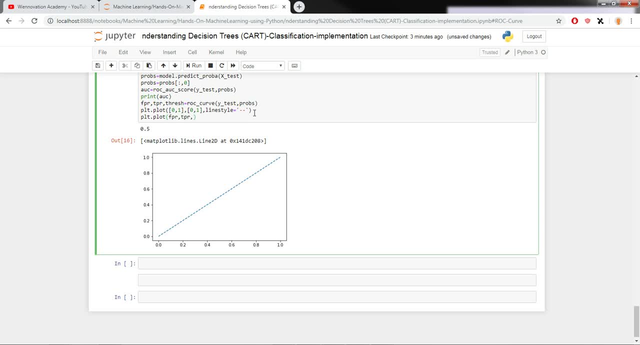 fpr, tpr and comma. so what is the markup here? so I'm just going to use a marker as equals to, let's say, I put a dot right here, okay, and if I do that you can kind of get the idea right here that well, doesn't just change the color here, because obviously we cannot get kind of 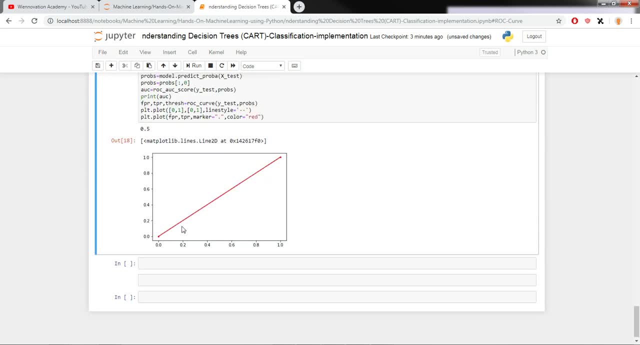 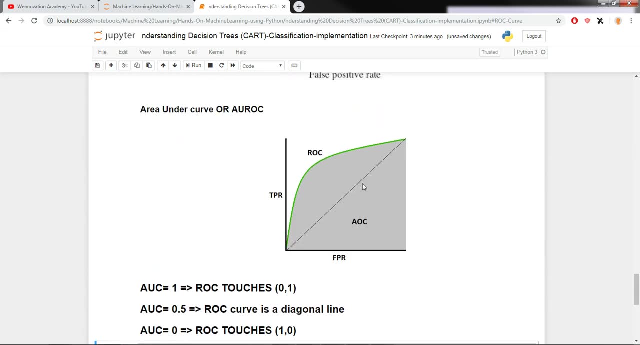 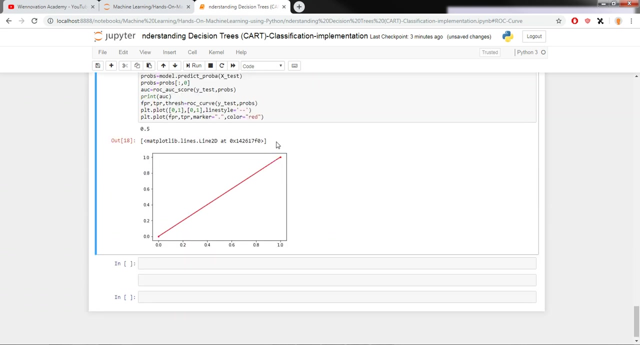 again the idea. here. I'm going to change the color to red and you can see. well, since we have the diagonal line on orange, you can see that this is exactly what we wanted to achieve, right? so you can see that the answer is simply a diagonal line, and we know that our model was simply incapable of you know. 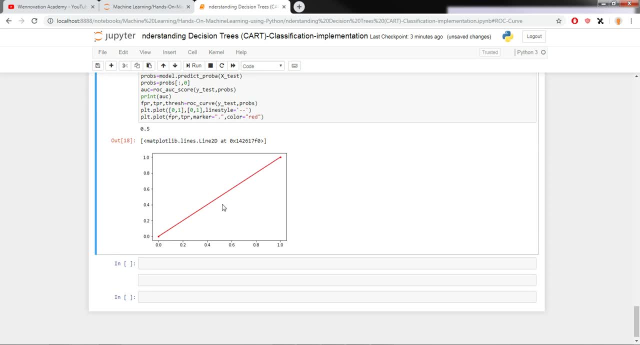 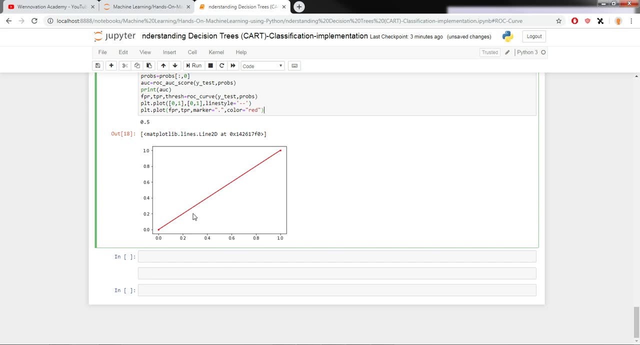 distinguishing between yeses and noes, and it's simply a random guess, right? so we obviously need better data and more data, right? so this is how you actually go ahead and draw an RC cup. now let me just go ahead and give you a very quick example of how we can actually go ahead and do this for for a bigger data set.